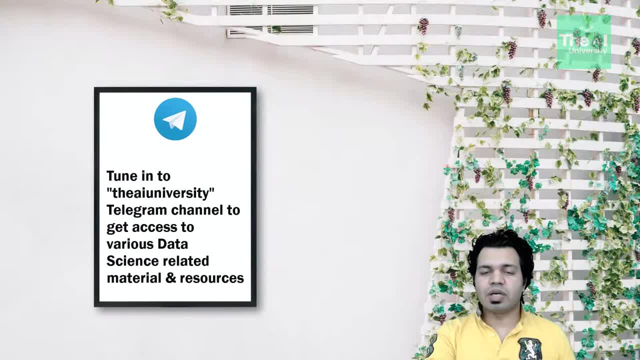 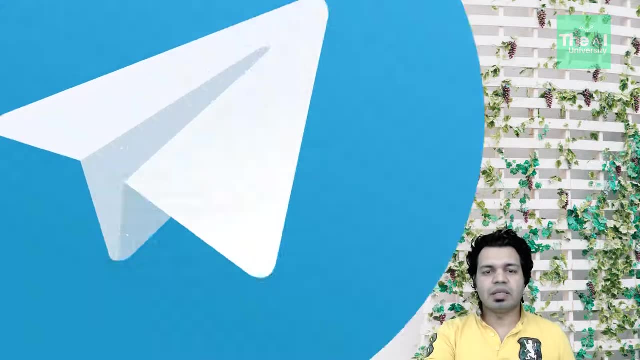 First I will give you a brief introduction of what are various pre-trained models, what is the benefit of using these pre-trained models, and then I am going to show you how to replace an existing VGG16 model layers with our own layers using Python language. 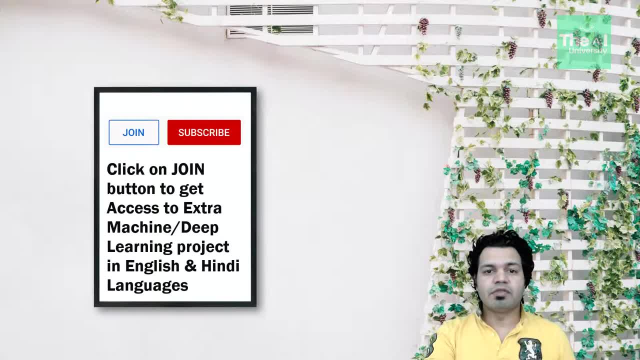 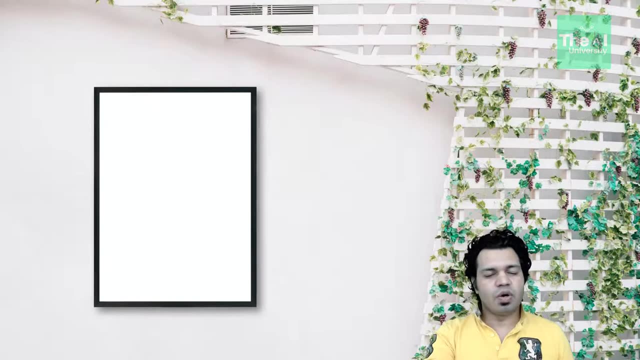 This can be a long video, but believe me that the information covered in this video will benefit you in long run, from the perspective of not only gaining knowledge on how to tweak an existing pre-trained model, but also giving an edge on other fellow data scientists. So watch this video till the end. 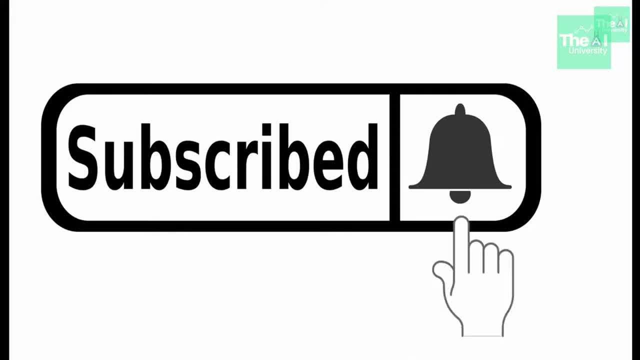 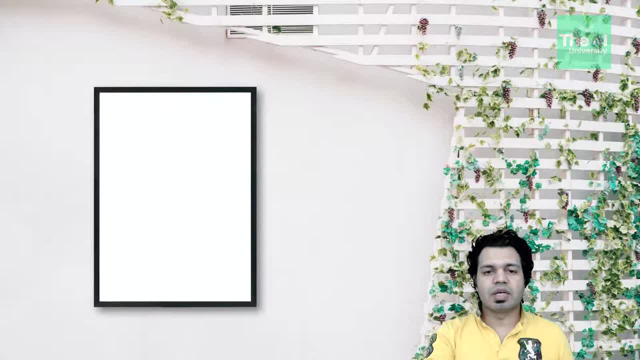 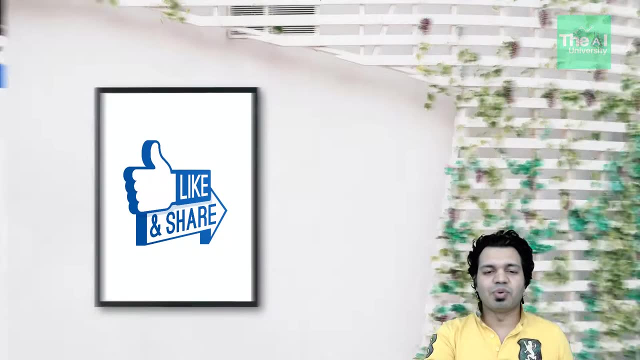 If you are new here, then consider subscribing to this channel, or if you have already subscribed, then click on the bell icon to receive the notifications about hottest technologies of 21st century. Please show your love and support by liking, sharing and subscribing to this video, as I will feel highly motivated. 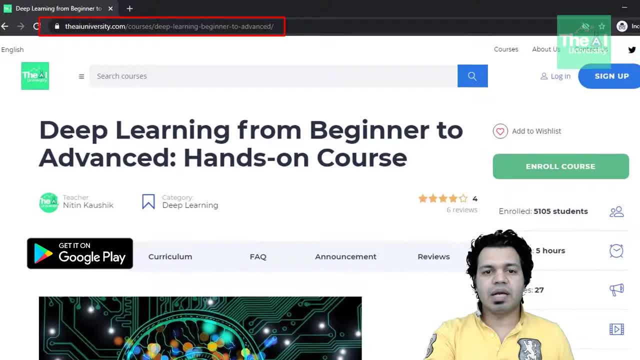 Also, we now have the AI University Android app and the website, which is in beta mode. You can download the code-related Jupyter Notebooks by enrolling to this course right here on the AI University website. All the courses are offered free on this website. 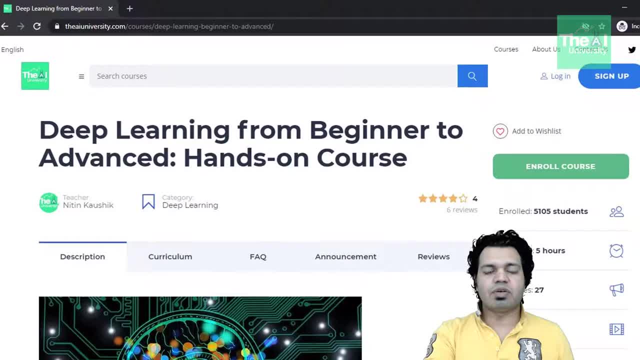 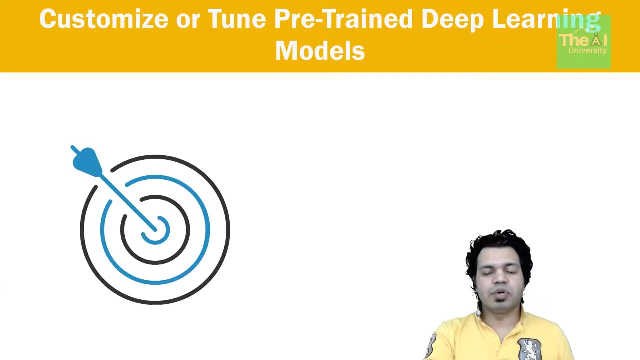 You can access the related quizzes and certificate of course completion like this, from the website once I upload all the videos. So let's move on. We know that if we want a machine learning or deep learning model that gives the best accuracy, then we have to train it on very large datasets. 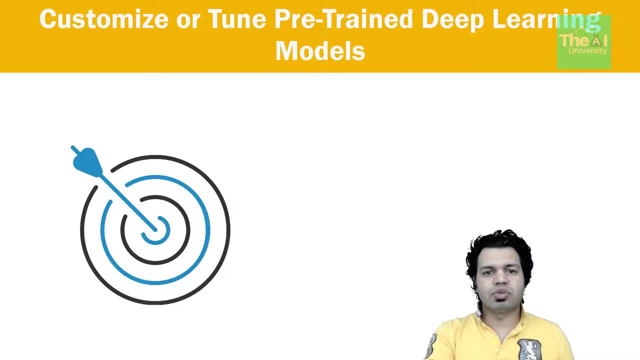 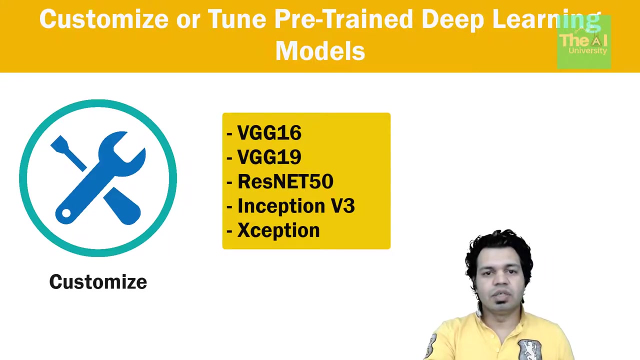 Deep learning models, such as convolutional neural network models, may take days or even weeks to train on the large image datasets. Now, if we want to cut short this high model training time, then we can make use of pre-trained model such as VGG16,, VGG19, ResNet50, Inception, V3, and Exception. 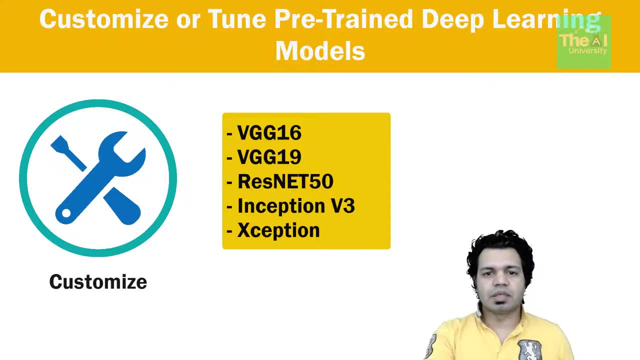 And some of them are trained on the ImageNet dataset. These models were developed for the ImageNet competition and built to predict one of the thousand different classes from, let's say, car to a man. There are several other categories involved in those thousand classes. 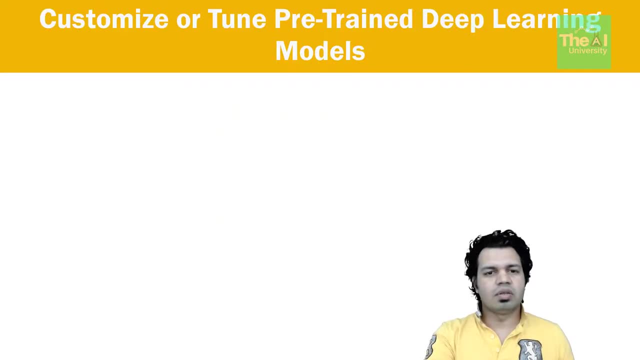 Maybe you know some household items or different kind of vehicles, etc. These were trained on millions of images, so the parameters associated with the convolutional filters are very well estimated. As I mentioned earlier, VGG16 is capable of recognizing thousand different object classes or categories. 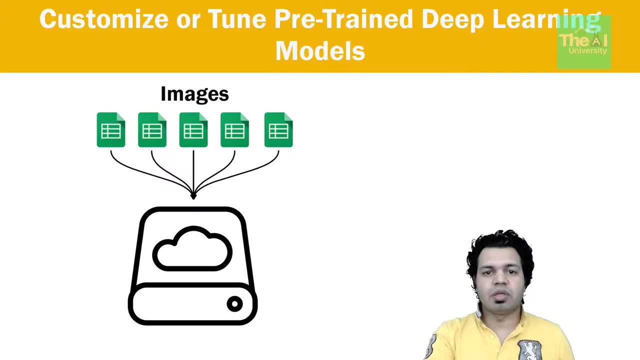 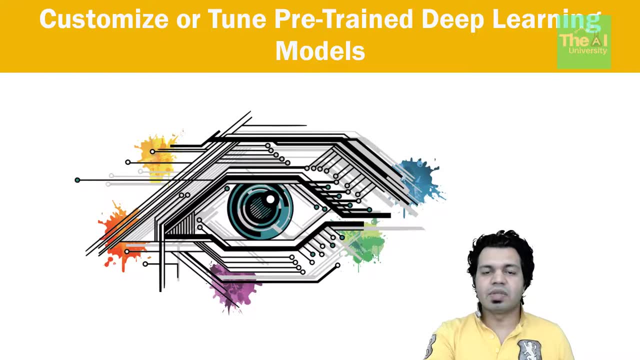 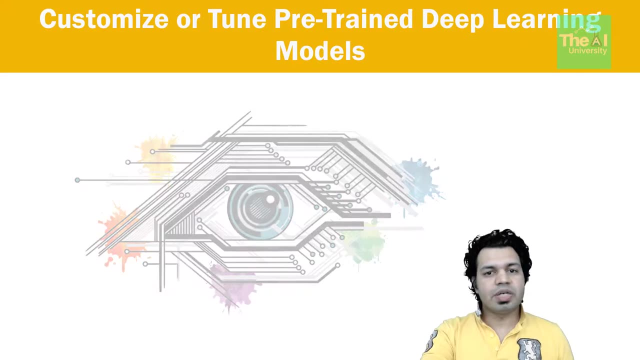 In a nutshell, we can say that we can reuse the model weights from pre-trained models that were developed for computer vision benchmark datasets, Such as ImageNet ImageRecognition Task. Let me also quickly tell you about ImageNet. So ImageNet in the context of computer vision or convolutional neural network? 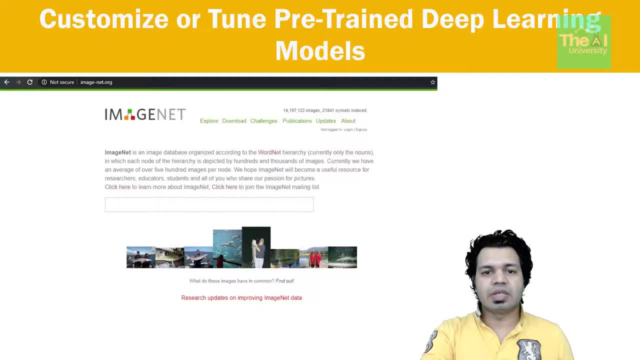 is referred to as ImageNet Large Scale Visual Recognition Challenge, or ILSVRC for short. This image classification challenge or competition, was aimed at developing and training a model that can correctly classify an input image into one of the thousand object categories. These thousand image categories represent object classes that we encounter in our day-to-day lives. 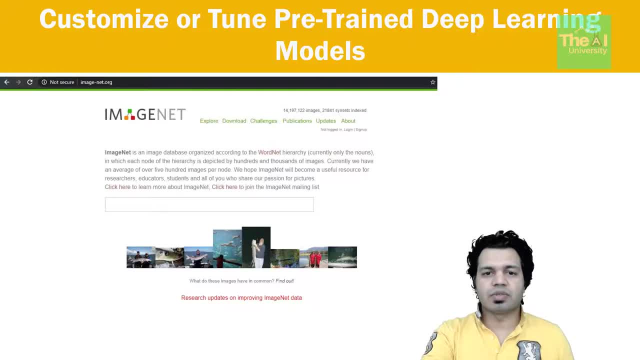 such as animals, vehicles, household items, etc. As a part of this challenge, VGG16 model got trained on whopping 1.2 million training images, with another 50,000 images for validation and 100,000 images for testing. 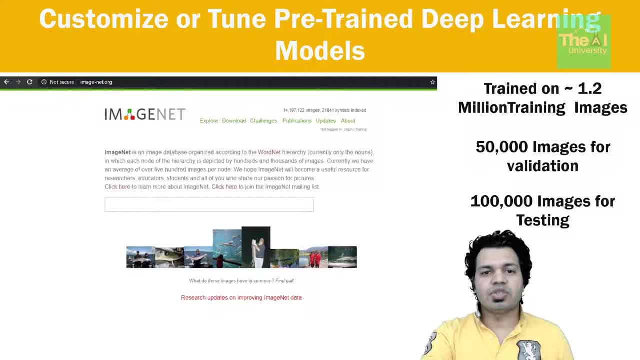 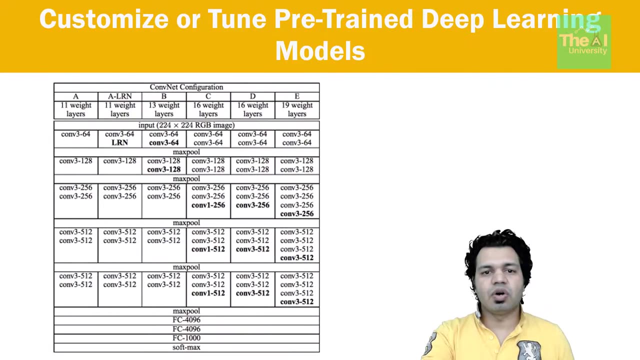 If you want to know more about ImageNet, then you can go through this website. I will provide the link in the description section. Now let's learn about VGG16 by going through its architecture. So VGG16 architecture uses 3x3 convolutional layers stacked on top of each other. 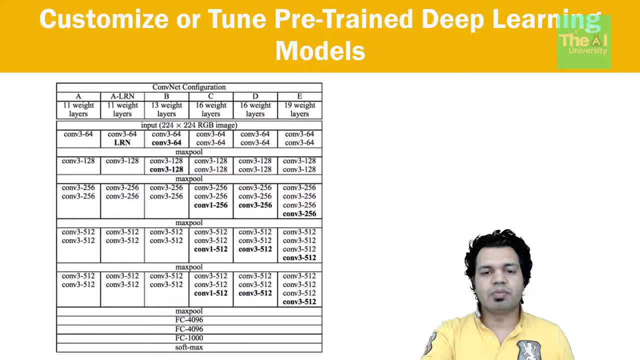 along with some other layers like max pooling, fully connected layer, softmax, etc. in the increasing depth. You can see this on the screen, which rightly depicts the VGG16.. As you can see here, the last layer is softmax class. This is a classifier that has thousand nodes depicting thousand classes. 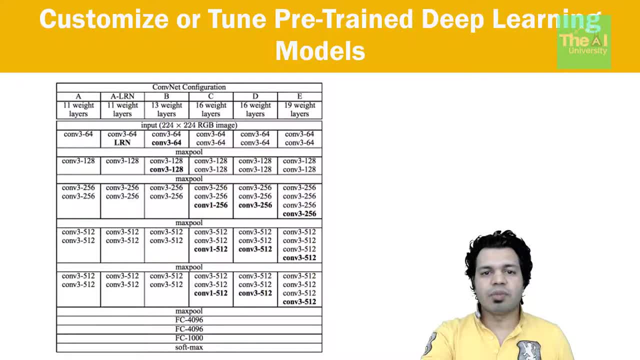 We will be removing this layer and replacing it with our own softmax layer containing only two nodes to classify only two classes. We can either download and use these models directly or customize it into a new model, as I mentioned earlier, for our own computer vision related problems. 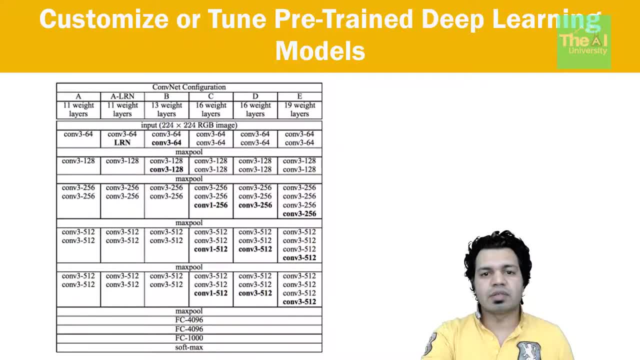 That is, to predict a custom group of classes. we can remove the final layer that depicts thousand output classes from this VGG16 pre-trained model and can add our own custom layer that contains only two classes. So essentially we can utilize these state-of-art networks in our own classification projects. 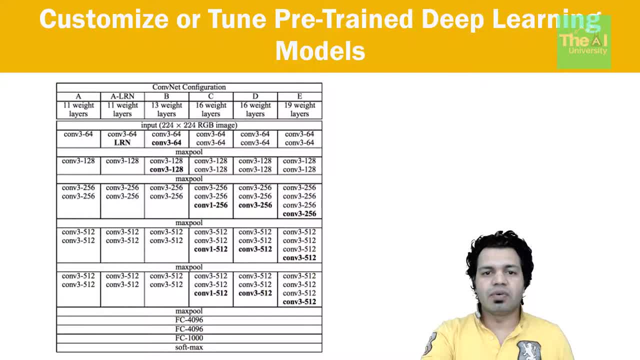 You will be glad to know that all of these VGG, ResNet, Inception and Exception network architectures are included in the Keras library And you can directly download them using Keras, And I am going to show you how. Now, if you are wondering what the number 16 and 19 in VGG16 and VGG19 represents, 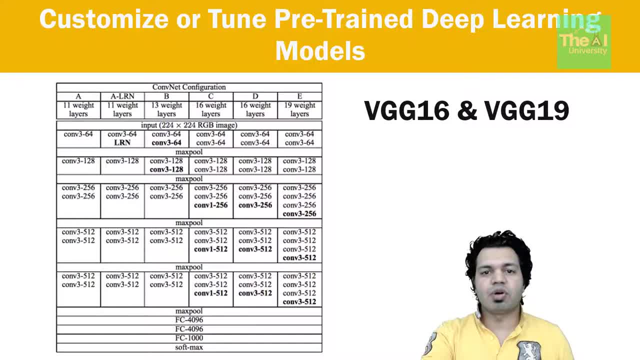 then I must tell you that these numbers represent number of weight layer in the network. as shown in the image, Column D represents 16 layers of the VGG16 and column E represents 19 layers of VGG19.. You can count the layers for yourself to validate the number of layers. 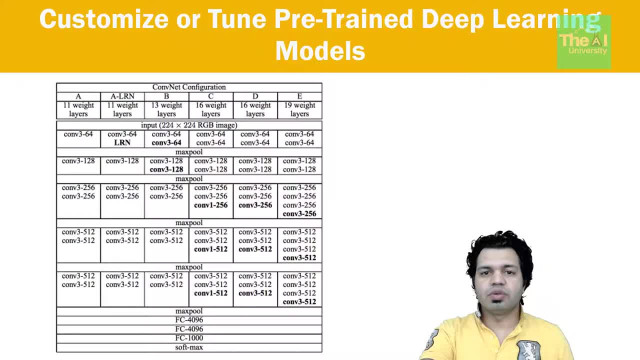 The VGG network architecture was introduced by Simone, Yann and Zizerman in their paper in the year 2014.. So, in a way, you are using model trained on one problem, but you are using it for your own unique problem. 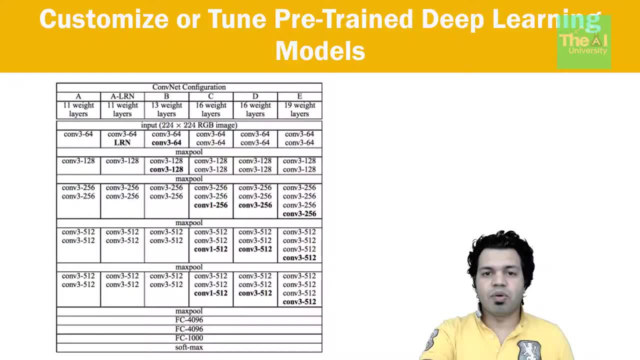 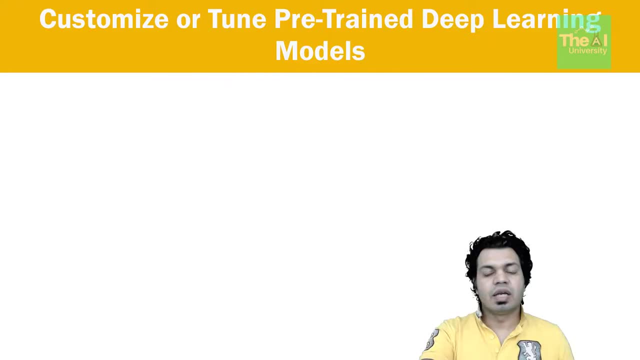 So this process, where a model trained on one problem is used in some way or the second related problem is called as transferred model. So remember that. Now let me move ahead and customize an existing VGG16 that can classify only two classes. 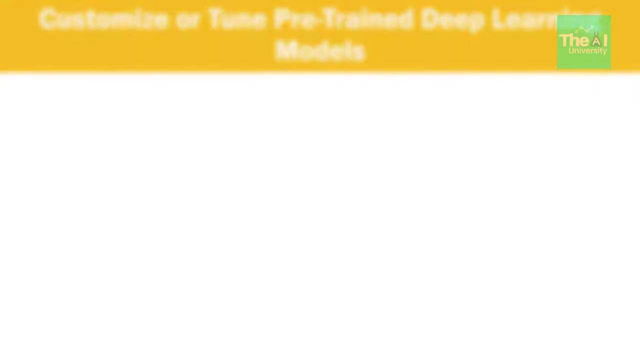 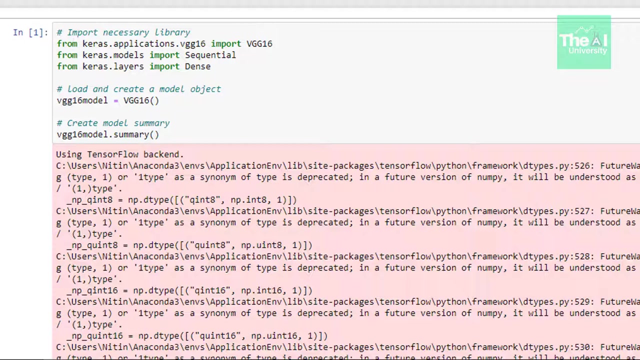 such as car and aeroplane, instead of thousand classes. So let's now open the Jupyter notebook. As I told you earlier, Keras provided these pre-trained models. So first we are importing our VGG 16 from kerasapplicationvgg16.. 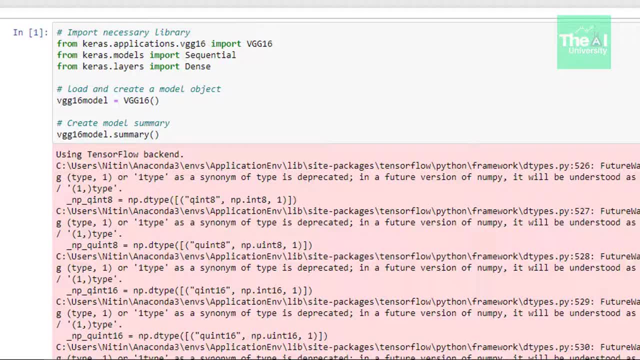 You can download other pre-trained models Like this only as per your need. So whenever you load these pre-trained models, the associated weights are also downloaded in your computer. In the next line, we are creating an object of VGG class and storing it in a variable called as VGG16 model. 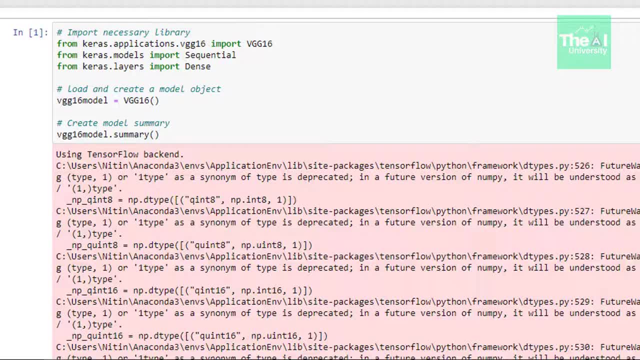 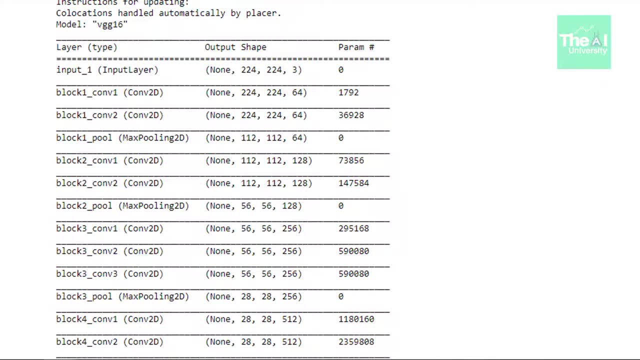 In the next line, we are generating the summary of model by making use of summary method, So let me show you. So here you can see the summary where you can observe the several layers, The layers associated with this VGG16 model. 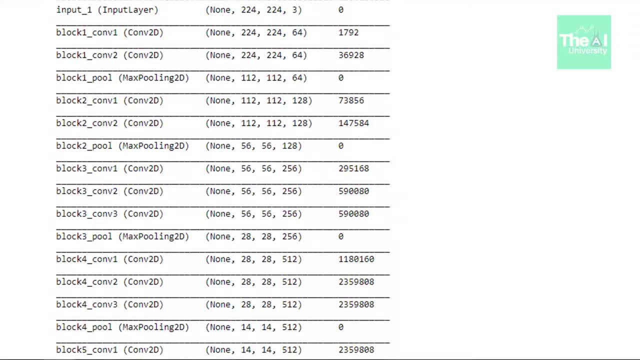 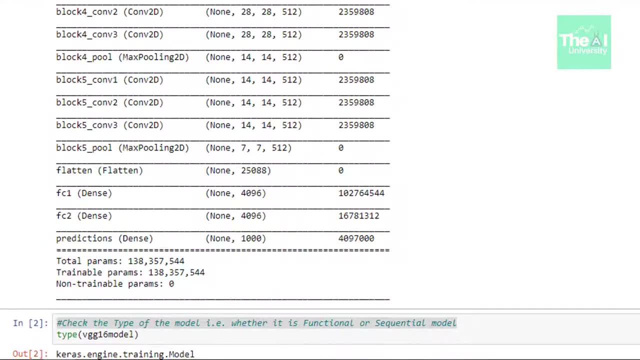 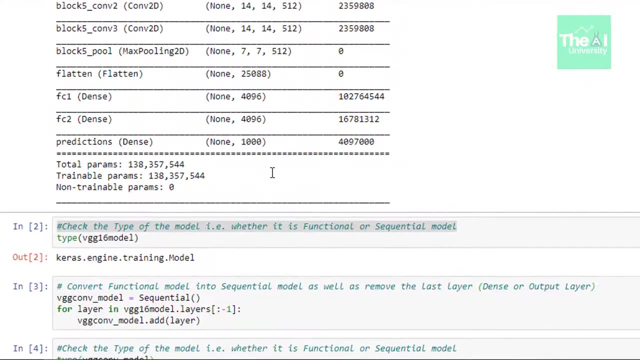 So here we have several convolutional layers, max pooling layers, fully connected or dense layer, Right. So just scroll down and you will see various layers stacked on top of each other. And now let's see this last layer here. 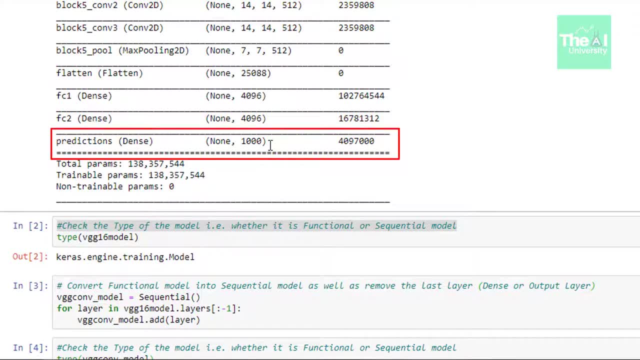 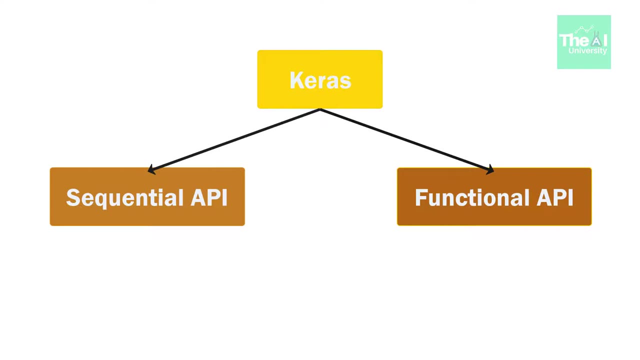 You can see that it has thousand nodes or separate classes or categories mentioned here, Right. So this is the first layer where we have thousand nodes. Right Now. this VGG16 model is a functional model And every model in Keras is either built using sequential class, which represents a linear stack of layers. 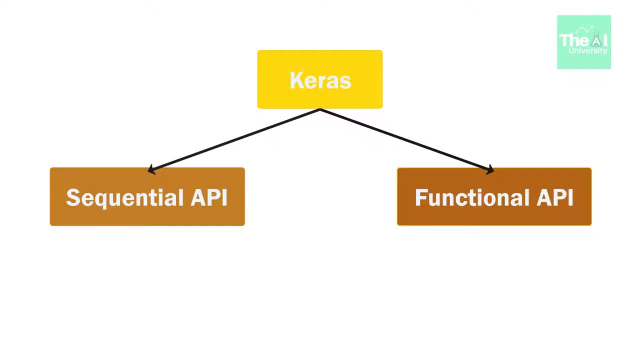 Or the functional model class, which is more customizable. The sequential API allows you to create models layer by layer for most of the problems. It doesn't allow you to create models that share a single layer Or have multiple inputs or outputs. Functional API, on the other hand, allows you to create models that have a lot more flexibility. 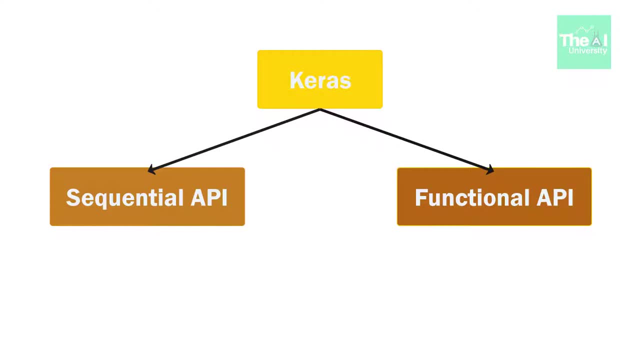 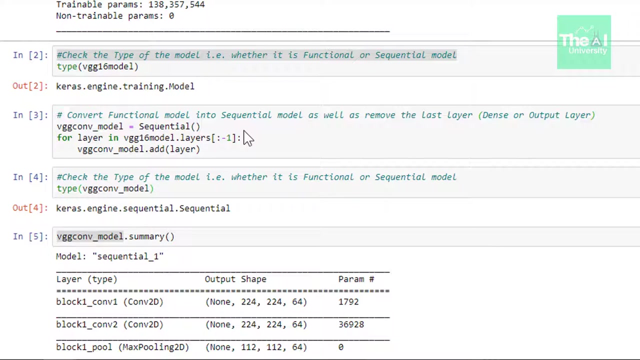 As you can easily define models where layers connect to more than just the previous and next layer. So our next step is to convert this functional VGG16 model to sequential model, Because sequential models are more simpler. You could validate if a given model is sequential or functional by making use of Python's type function. 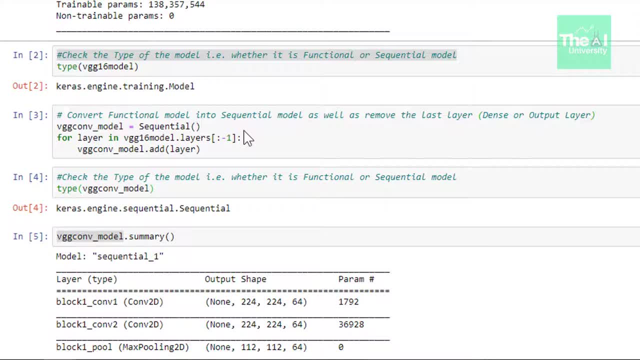 So in the next cell we are checking that. only When we ran this cell we got the output as kerasenginetrainingmodel. So here value model represents that it's a functional model. If this model is sequential, then it would suggest that it's a sequential model. 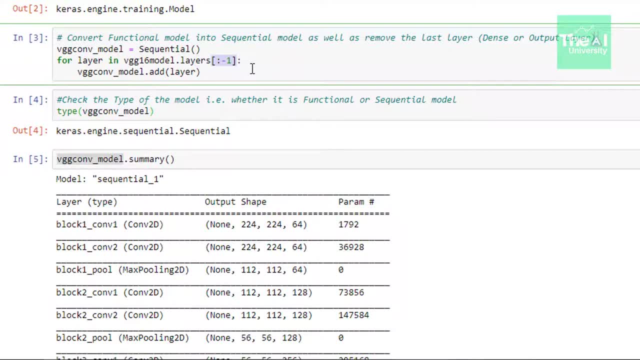 So let's move on to the next step. Let's move on to the next cell where we are converting this functional model to the sequential model. So first we are creating an object of keras sequential model And we are referring that object as vggconv__model. 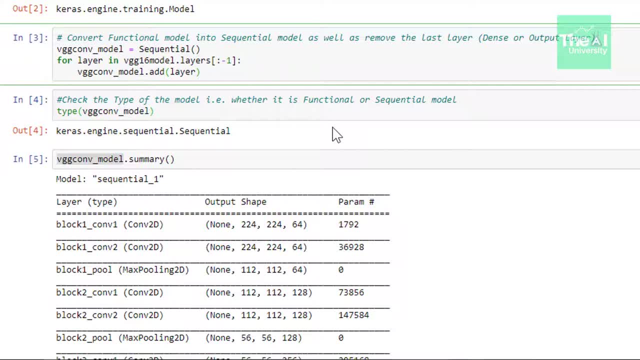 In the next line we are making use of for loop to iterate through all the individual layers of the functional model And then adding those individual layers to the sequential model named as vggconv__model. So when we defined vggconv__model as sequential right here, it didn't have any layers. 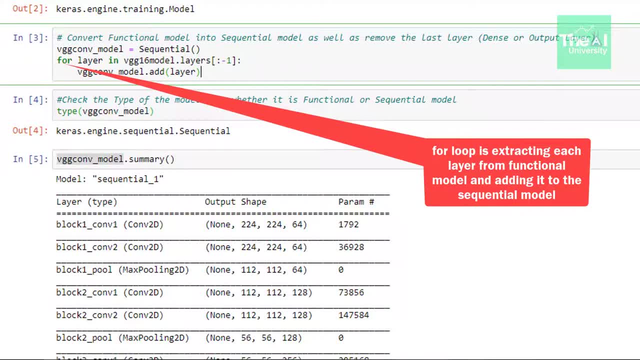 It is the for loop which is adding layers to our sequential model. This way we can convert a functional model to the sequential model. Now we are doing one more thing here: We are also removing the last layer from this sequential model which we are building here. 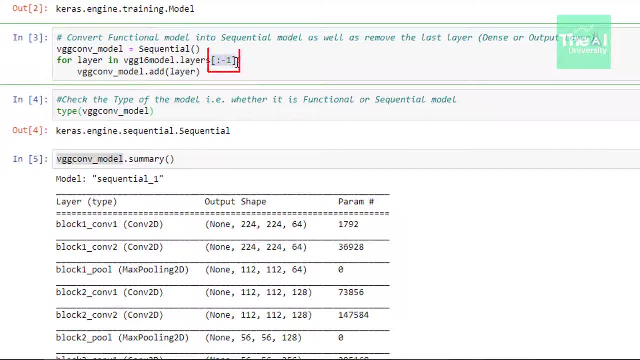 So we are removing the last layer using this, This particular subscript, which is colon minus one, inside this solid brackets. So what it will do is it will just remove the last layer from this model. In the next cell, we are just checking the type of this model. 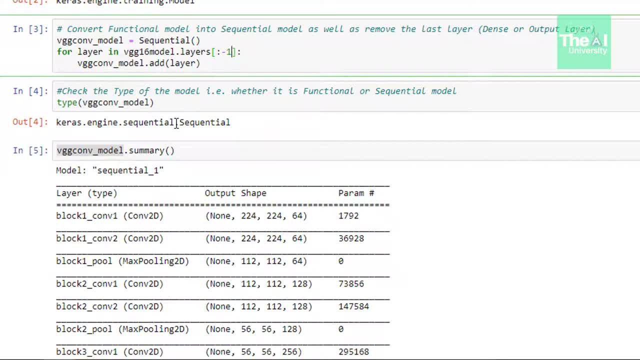 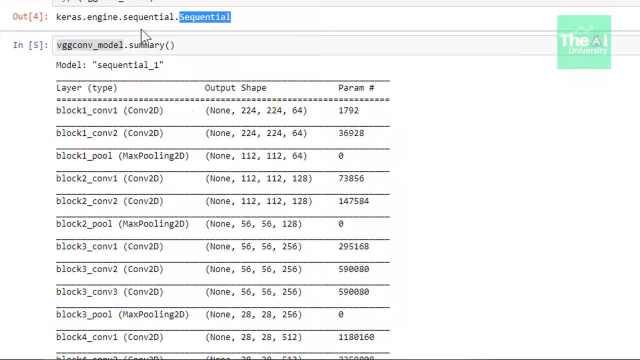 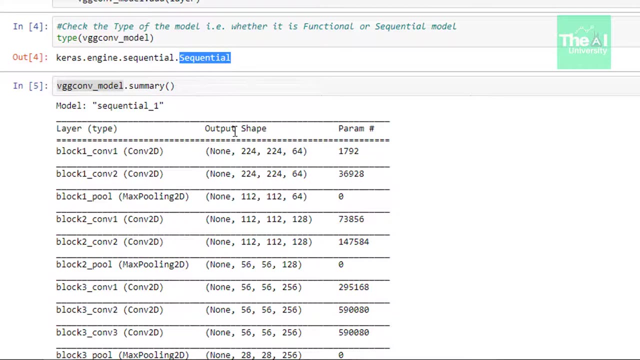 You can see that this is shown as sequential here now. Next, I am just showing you the summary of this new built model. In the next cell I am showing you the summary of this model, which is converted from functional to sequential model, to show you that last layer has been removed. now 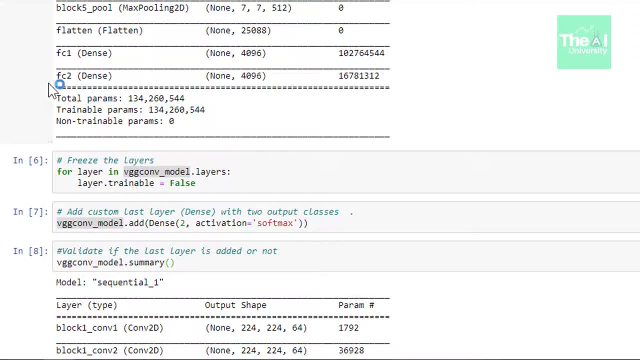 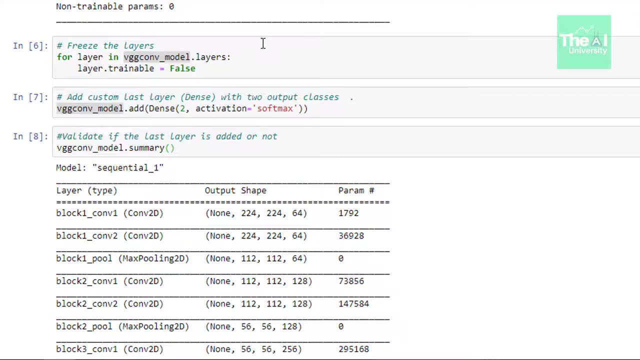 So you can see that last layer has been removed. now There is no dense layer with thousand nodes. here In the next cell, we are using for loop to go over each of the layer of our sequential model and then setting the layertrainable parameter as false. 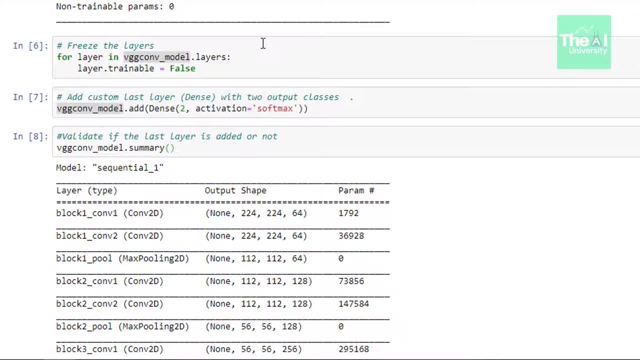 Now the question arises: why are we doing that? Well, we are, in a way, restricting the layers for future training so that weights doesn't get updated. This is being done because the weights that we got after VGG16 model got trained on millions of images- are optimum. 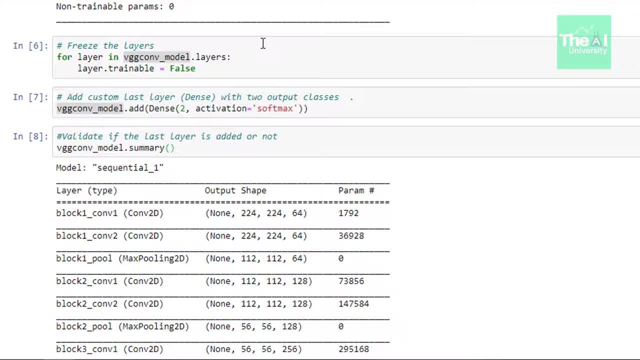 Let's say you train this customized model on 50,000 images now. So you will get some weights that might be inferior to the ones associated with the original VGG16 model, And chances are you might not get the state of art accuracy. 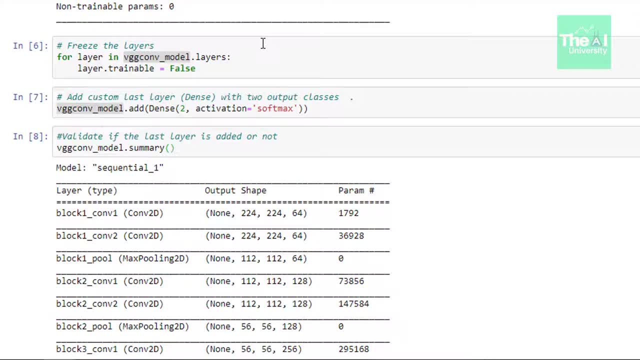 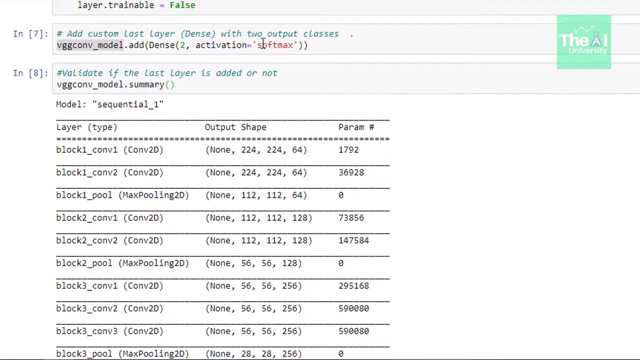 as you got on VGG16 model, But if you have some unique requirements, then you can very well skip this step. Finally, in the next cell, we are adding our own dense layer that contains two classes: one for car and one for aeroplane. 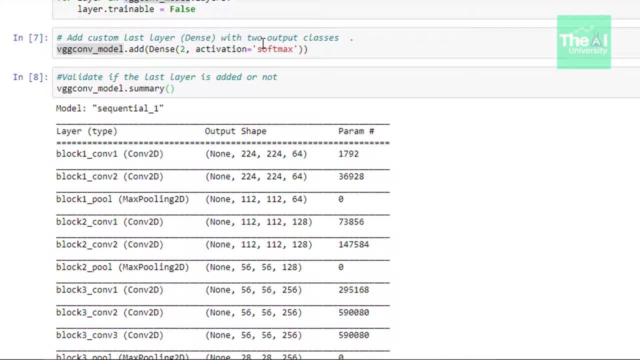 So we are adding a dense layer here, passing number 2 right here as an argument and which signifies the two categories or classes Moving on. So activation function being used here is softmax. So instead of thousand nodes, so instead of thousand classes. 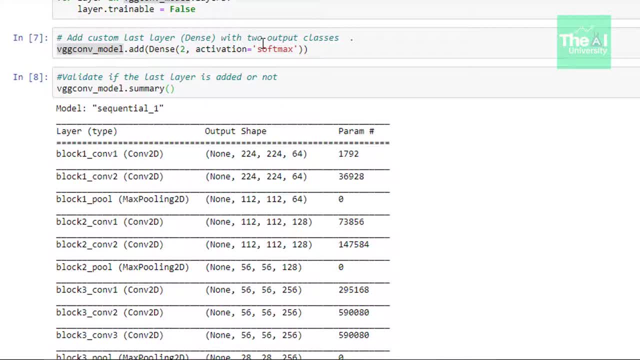 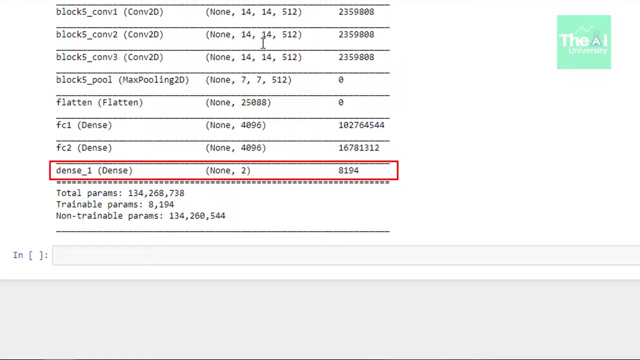 only two classes will be predicted by this model. now In the next cell, we are generating the model summary to see the various layers or structure of our customized VGG16 model. Let me scroll down So you can see that the model now has the output layer that we have added. 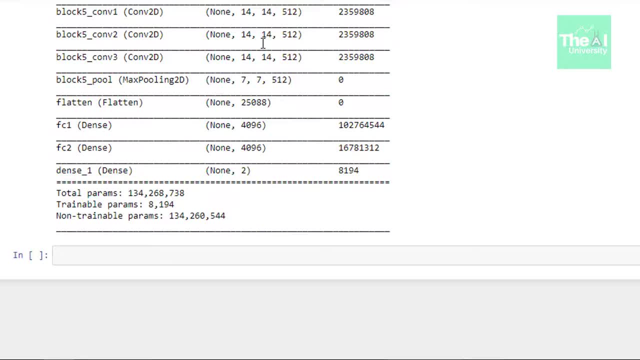 It has two output classes or the two nodes here. So this is the way we can customize any pre-trained state of art model according to our need. We can customize it to predict 10 classes, or maybe 25, or maybe many more. So hope you have learned something new today. 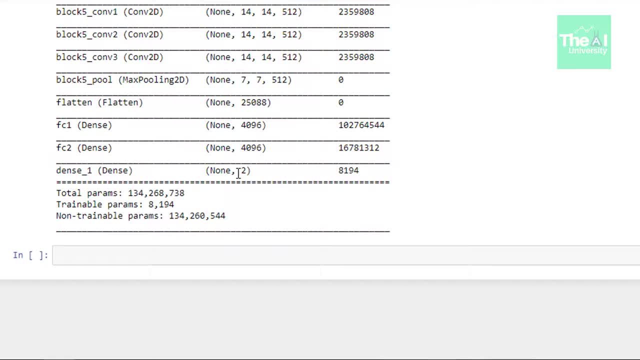 So, folks, this is it for this video. In the next upcoming video, I will cover another important topic. So here is today's question. Using the concept or the steps shown in the video, you can tweak any existing pre-trained model. 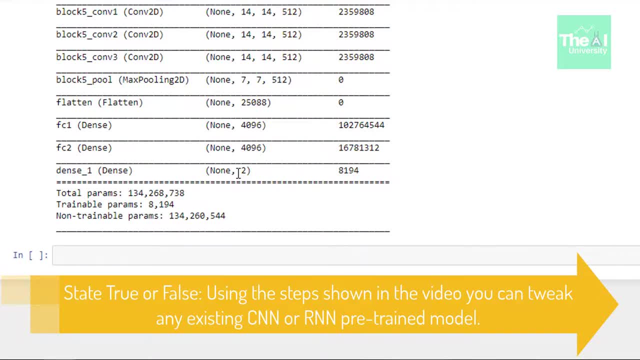 be it recurrent neural network or convolutional neural network. Please post your answers- comments- in the comment section given below, so that I can get a chance to incorporate your feedback. You can also post your technical questions in that comment section and I will try to answer the same. 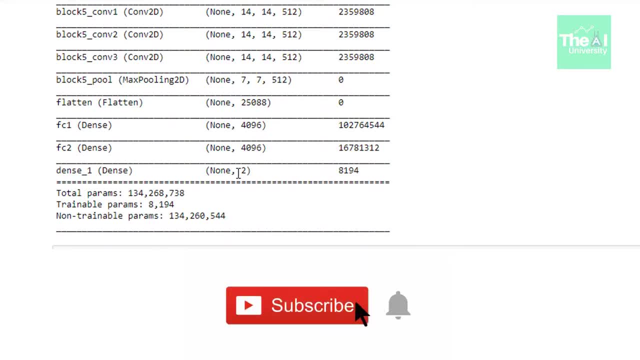 If you are watching this video and you are not already a subscriber to our channel, consider clicking that little subscribe button. In case you have already subscribed, then click on the bell icon to receive the notifications whenever I will release a new video. So thanks for hanging out with me, guys.